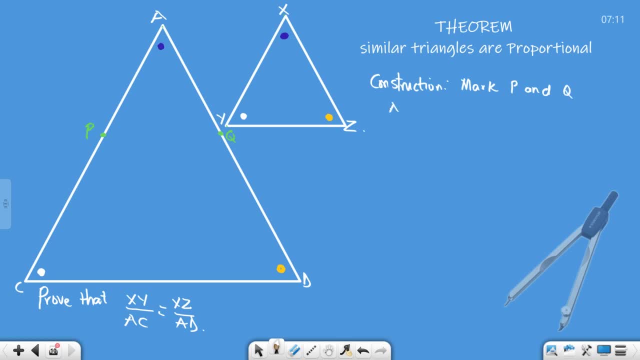 Okay, Such that. a Okay mark off p and q. Um join p- q. but I think such that let's write this such that: what a p is equal to x y and a q is equal to x- z in length. 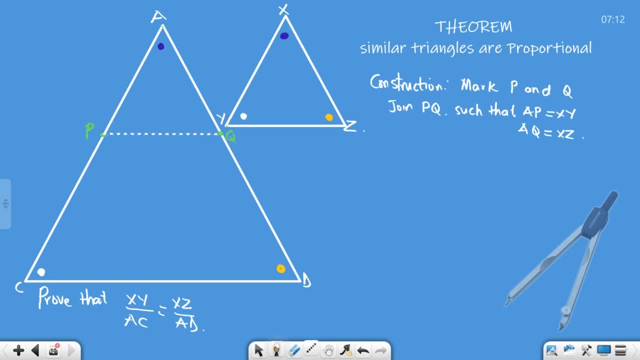 So I am just going to join that now. All right, So we are saying: this should be equal to that. This should also be equal to that. Sweet Already. I have been able to bring that triangle over to that side. So that's the first thing we have marked off our point. 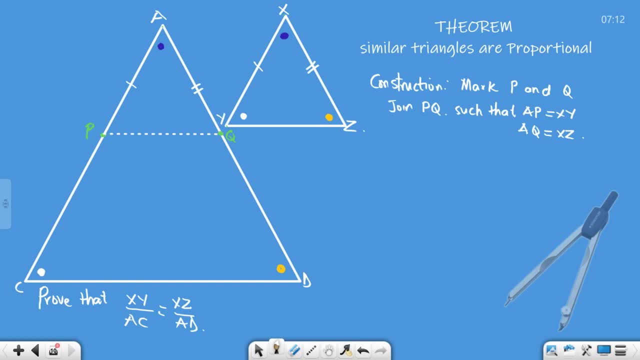 We have joined. but let's see Now. if I look at this check, I'm going to consider, so that you remember, consider the new triangle: triangle a, p, q and triangle What, X, y, z. 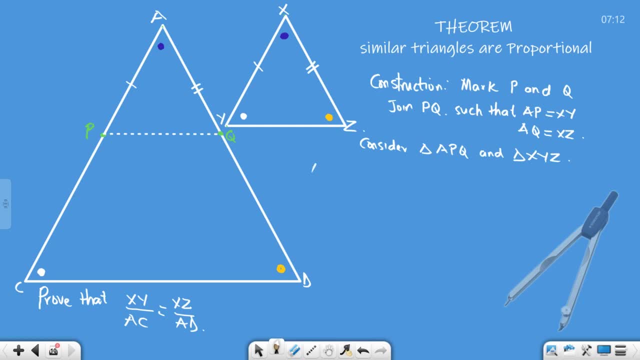 Remember: a p is equal to x y by construction. A p equals to x y by what Construction? That's a side already. Angle a is equal to angle x. We are given the blue one. Now the other side, a q is equal to x, z. also by what? 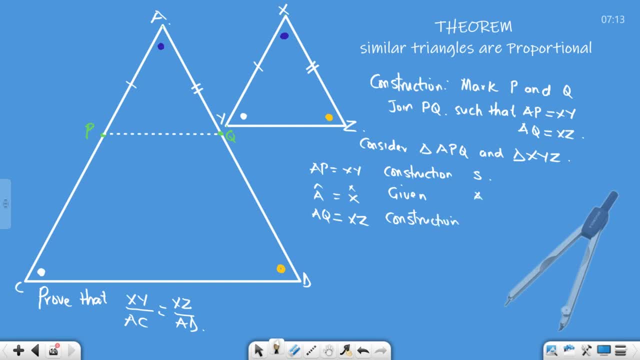 Construction. Now what have we proven? Oh, we have proven that they are congruent side angle side. Therefore, triangle a, p, q is congruent to triangle x, y, z. That's very important. The order: 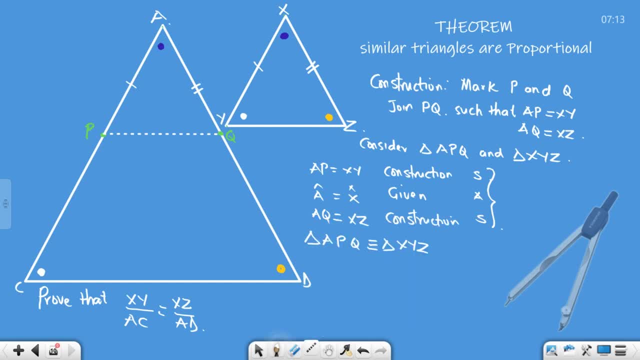 Let me get a highlighter. The order is very, very important. We have proven that a, p, q is congruent to x, y, z. That's very, very important. It therefore means check what we've done. 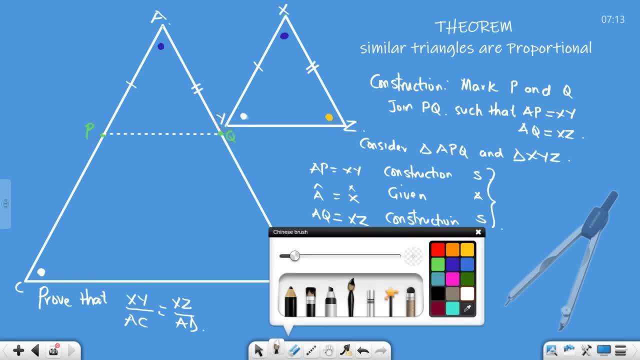 We have transposed this angle. This angle is now here. the white one, Oh sweet. The yellow one, because we are saying these triangles are exactly- no, that's not yellow, are the same, Oh sweet. So we can then now say that angle p is therefore equal to angle c. 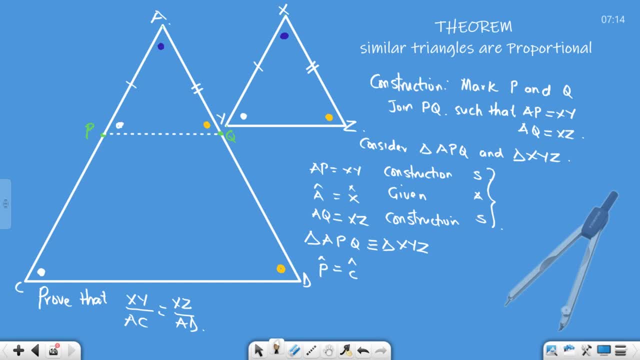 All right, Because we can see there: Oh, that's basically almost saying corresponding. Therefore, p, q will now be parallel to c, d. That's your aim, converse of corresponding. So we are now saying that this line and that line are parallel. 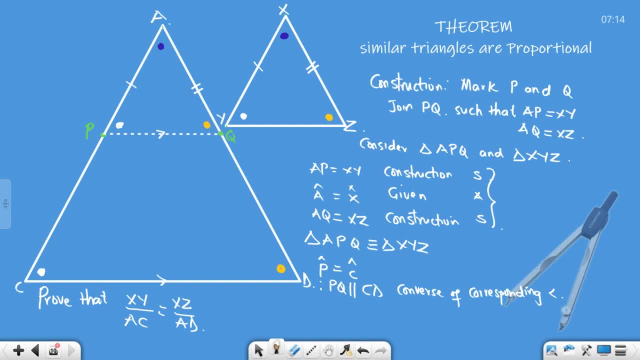 And once you have that, we can then use our proportionality theorem. You don't need to prove proportionality, You have already proven that those are parallel. Now remember we are proving x, y and a, c, which is the top. 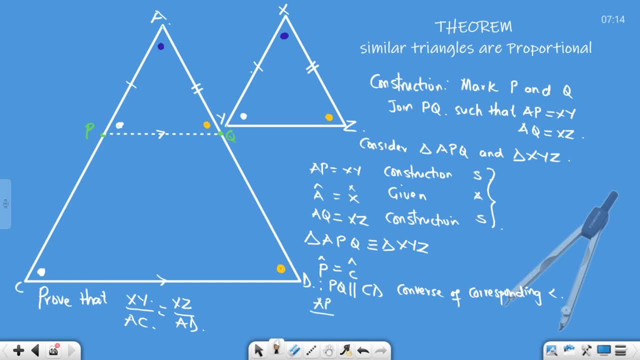 Therefore I can say: a p over a c is equal to the top. again on the right-hand side, a y over a d. What's your reason? Proportionality, what The theorem And which line is parallel? 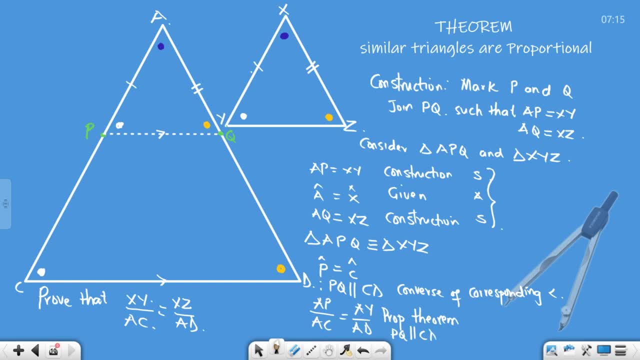 You are saying that p- q is parallel to c- d. By the way, do you remember that a? p is equal to x- y by construction, And a? y is equal to what x? z, also by construction? All right, 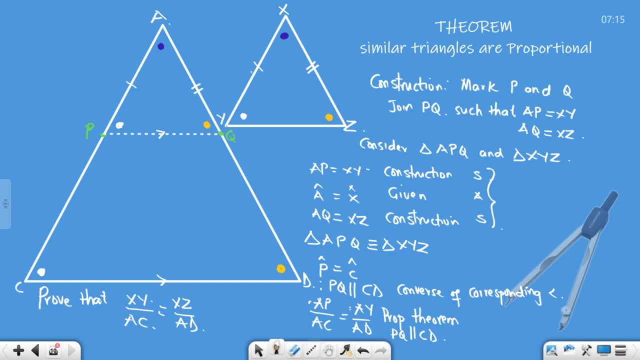 Oh no, I said a y somewhere should be a q. Okay, the triangles were too close. A q. Let me just quickly get rid of that. It's a q, Okay, so a p over a c a q. 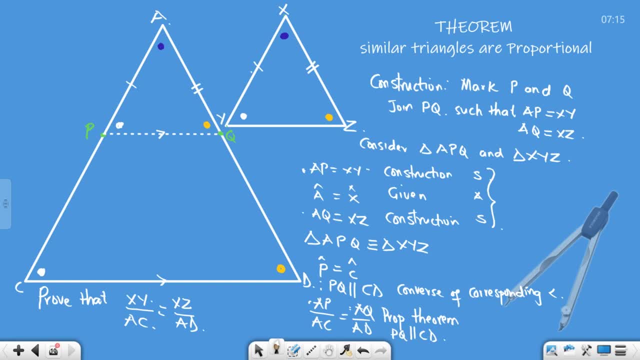 But I know my a p and my a q, My a p and my a q. Oh, it's x, y, and So we are done. Therefore, what is my a p? My a p is x y. 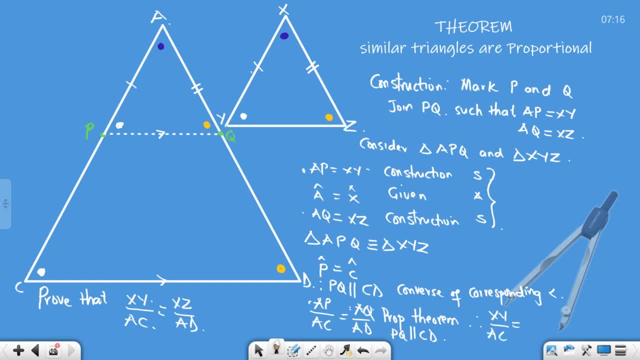 x y over a c is equal to What is my a q. Remember, my a q is x z Over what A d And we are done with the proof. So this is the last proof in grade 12, which you need to know before you get into an exam.